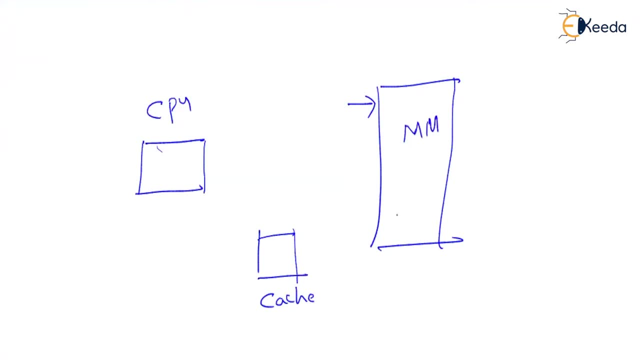 and this is main memory Spare, though the shape is not good, fine. Okay, now the CPU has a direct connection to the main memory and also CPU has another parallel connection to the cache memory. Okay, Main memory is accessed directly by the CPU as well as the cache memory, also connected to and from the main memory. 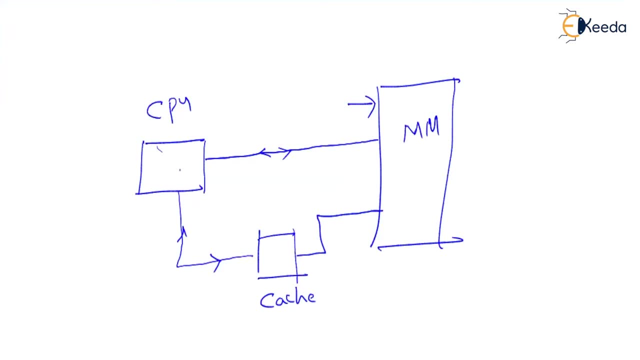 Now, initially, when a CPU wants to access a data element, okay, the data element could be either an instruction or an operator, as you already know. Okay, now, regardless of that, let us say CPU wants to search for a data element. Initially, the search will be: 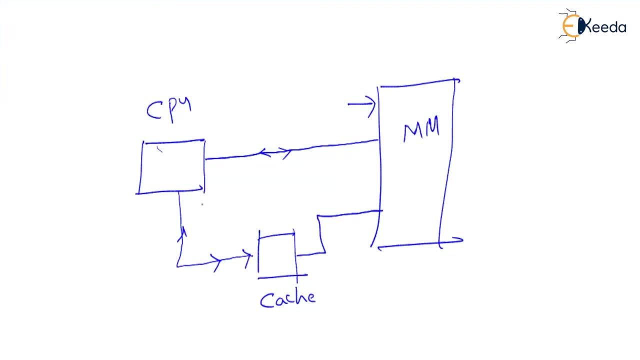 made in the cache memory. That means whenever a CPU wants to access a data element, initially for that data element cache will be searched. Okay, If cache has the data element, then the data element will be collected from the cache memory itself. Okay, If the cache doesn't have the data. 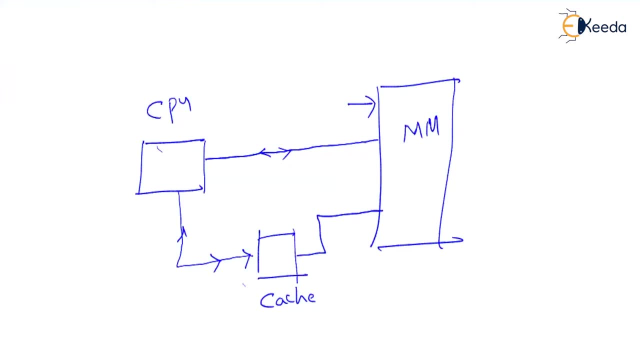 CPU is directly going to access main memory. Okay, Now stay focused. When cache has the element, then the data element will be collected directly from the cache memory. If the cache doesn't have the data element, CPU is going to access main memory to get the data. Now let us. 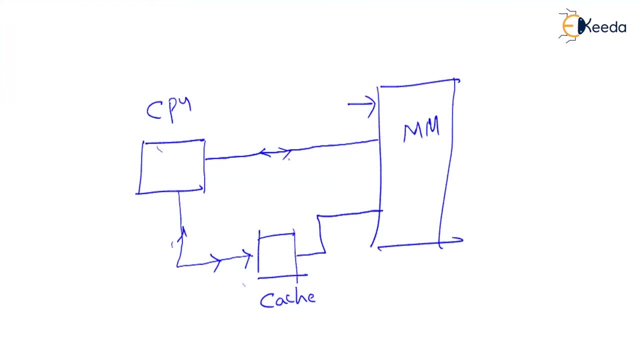 say during cache doesn't have the data element, main memory will be accessed and CPU will access this data. At this time, the corresponding data element will also be transferred to the cache memory. Why? Because the data element which is accessed currently can also be accessed in the 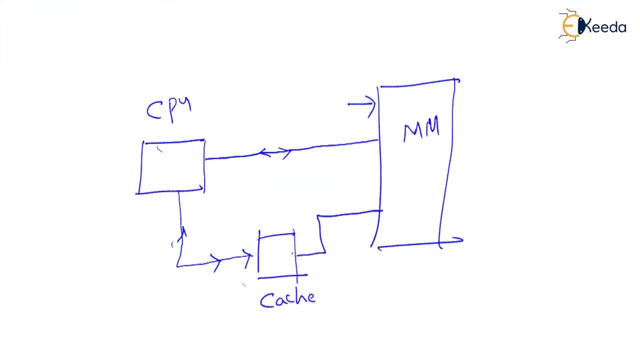 near future. This is the primary implementation logic of the cache memory. Okay, Now, this is how the cache will be accessed When it comes to the secondary memory. when it comes to the secondary memory, the secondary memory is connected beyond the main memory, because secondary memory is only. 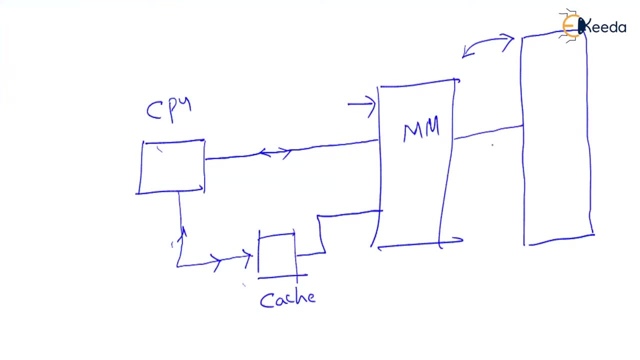 auxiliary device. Now let us understand the hierarchy here. When CPU wants to access the data element first, for the data element will be searched in the cache. If it is not available, I will go to the main memory and I will directly access it from the main memory. Meanwhile, the corresponding data element will also be 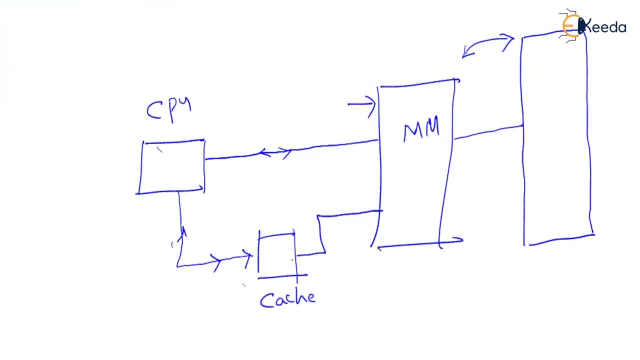 transferred to the cache for the future references. Okay, The element which is accessed currently might also be accessed in the near future. Okay, Now let us see. The data element which is being searched is neither present in the cache memory nor present in the main memory. So at that time, what CPU does? Can CPU directly go to the main- sorry, secondary- 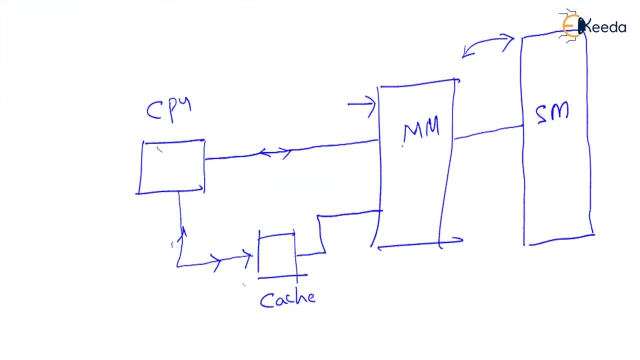 memory and search. No, You can clearly see that CPU. there is no direct connection between CPU and the secondary memory. Even though the data is not present in the main memory, CPU will not access secondary memory directly. Okay, Initially, if the data is not available in the main memory, the data element will get transferred from. 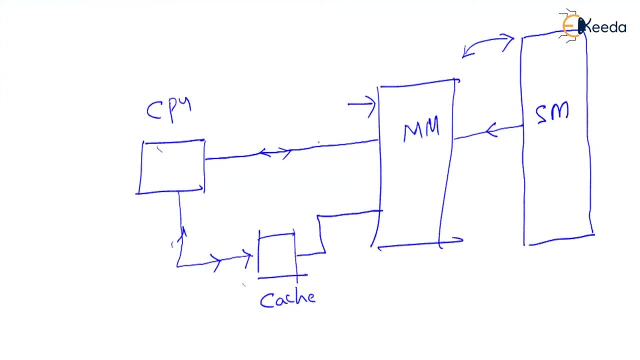 secondary memory to the main memory. Finally, the CPU is going to access any data element only from the main memory. That is the fundamental rule. CPU can never talk to the secondary memory directly. Okay Now, why CPU can't talk to the secondary memory directly? Let us see. Let us see that. 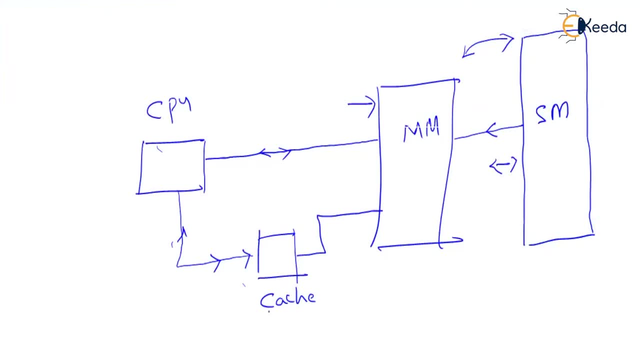 Let us consider that the cache memory���ijuana memory, will take one nanosecond, rather one clock cycle. Cache memory will take one clock cycle, That is, one clock cycle. I will say that clock cycle In order to seek the data element. 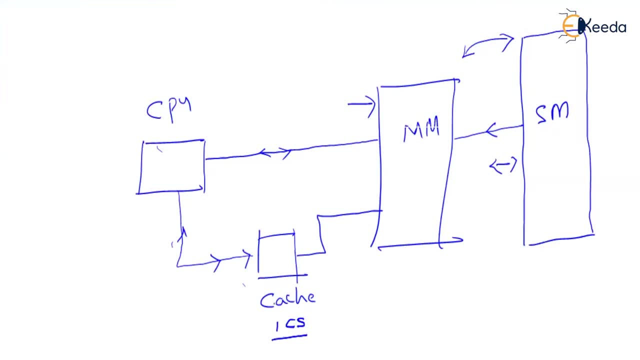 if the data element is present in the cache, then it will take one clock cycle to look back andfounder. Okay, that data element into the cache memory. okay, to access any element out of the cache memory, CPU just require one clock cycle if the same data element, if it is. 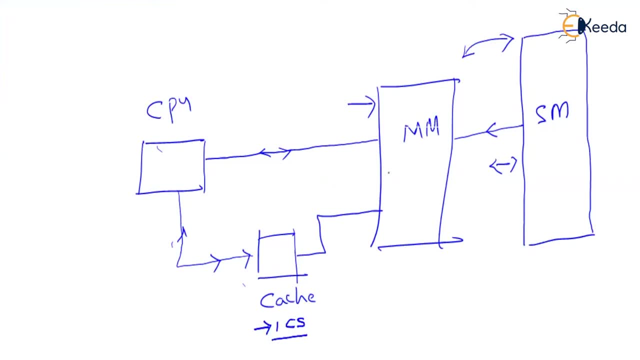 not present in the cache, CPU will have to go to the main memory and access it. so main memory will take seven clock cycles, seven clock cycles to locate and get this data element. the data element will take seven clock cycles to be located and fetched. okay, so the axis difference is one clock cycle is for the. 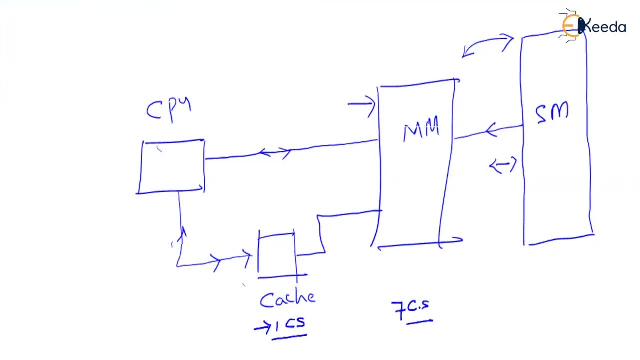 cache memory. seven clock cycle is for the main memory. now you can clearly see when cache doesn't have the data. the miss penalty will be one more clock cycle. you know what is miss, what is hit and miss what is hit. if the cache has a data element, it is a hit, what is a miss? the data is not present in the cache. 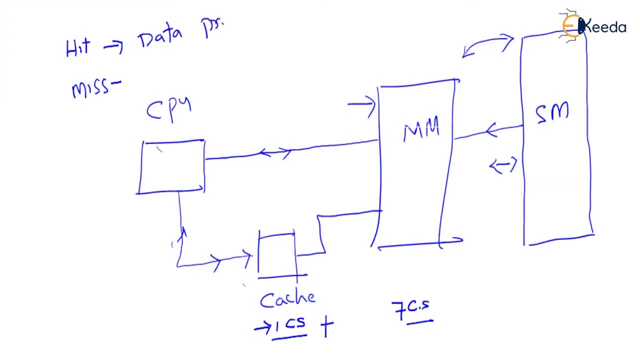 data present in the cache. data is not present in the cache. data is not present in the cache. okay, when there is a hit, CPU will directly read. when there is a miss, CPU will directly go to the main memory. got me now: in order to access mean memory for the data element, I do require seven clock cycle. so the access 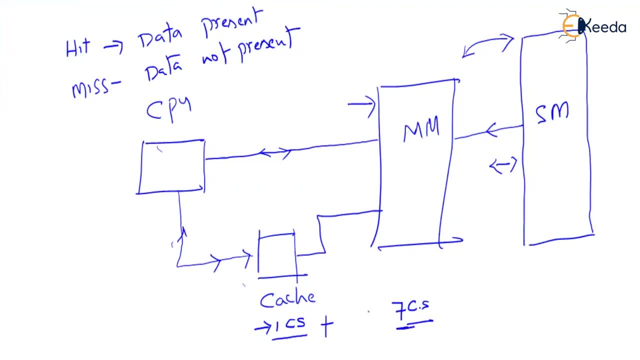 difference is seven and one. now the miss penalty will be: whenever there is a miss in the cachemary, then the miss penalty will be total eight clock cycle, because one clock cycle which is wasted at the cache memory will also be added to the total access time. so the total miss penalty will be eight clock cycles. that 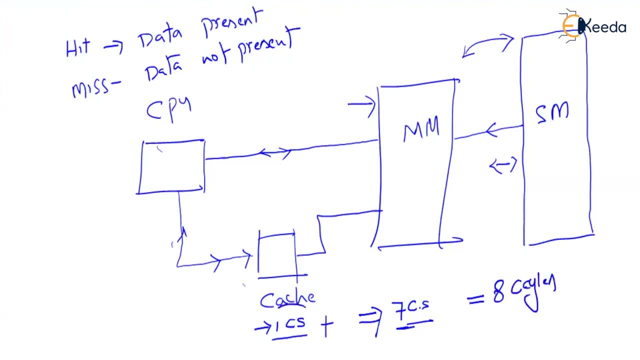 is the eight clock cycles, that is, a, The clock cycle which is wasted in the cache memory and the clock cycle that are required to access main memory. All together, eight clock cycles which are treated to be as miss. penalty: to access the data from the main memory whenever there is a miss in the cache memory. 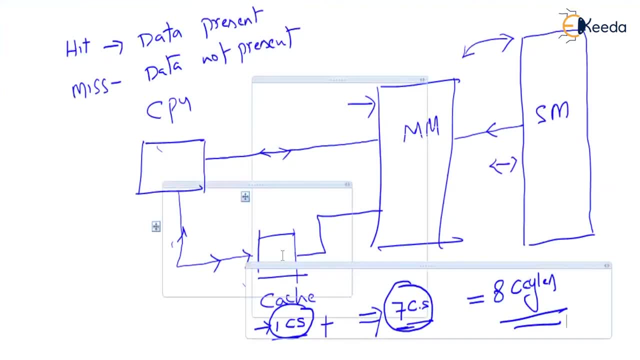 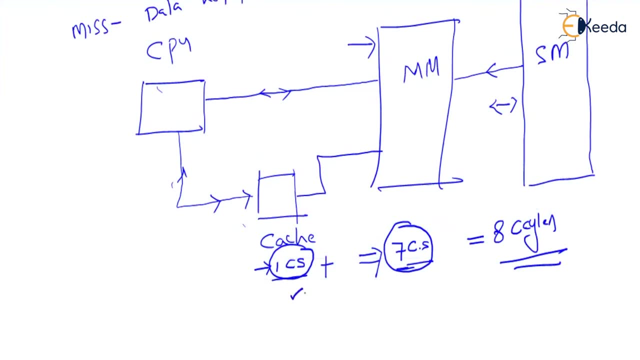 Now let us see why we don't, rather why CPU doesn't- access the secondary memory directly. You know that one clock cycle, all it takes is one clock cycle to access the data element from the cache. All it takes is seven clock cycles to access the data element in the cache in the main memory.